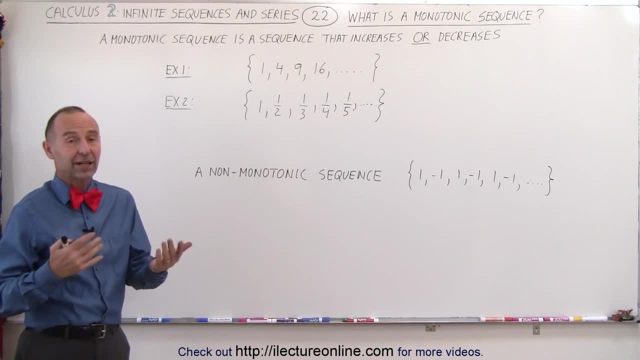 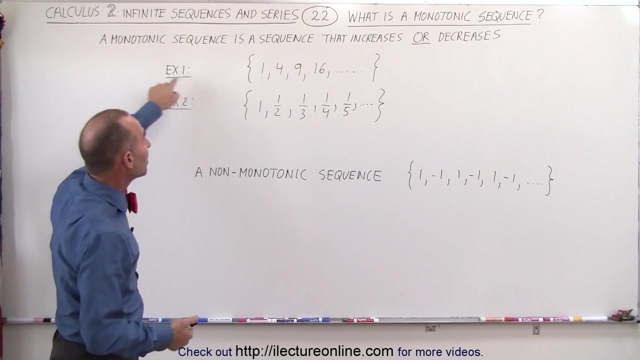 Welcome to iLectureOnline. Sometimes you'll see in a textbook a term and you have no idea what it means, such as a monotonic sequence. Well, it's actually fairly simple. A monotonic sequence is a sequence that either increases or decreases. Here we have an example of an increasing sequence. 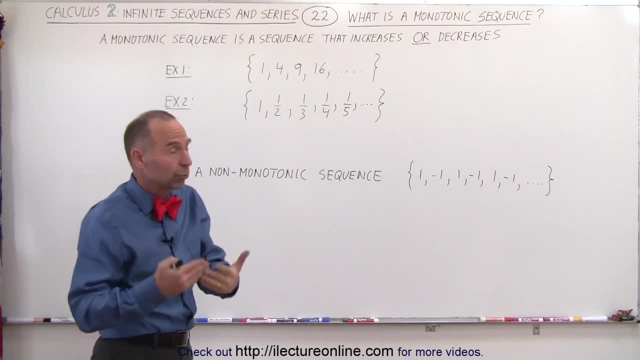 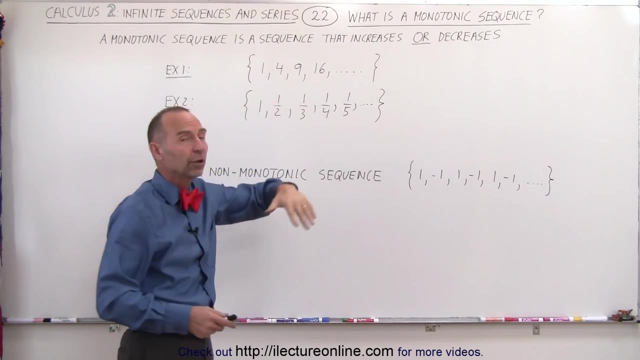 1,, 4,, 9,, 16, which, when you look at it a little bit more closely, you realize that this is the square of 1, the square of 2, the square of 3, the square of 4, and so forth. So you can see that. 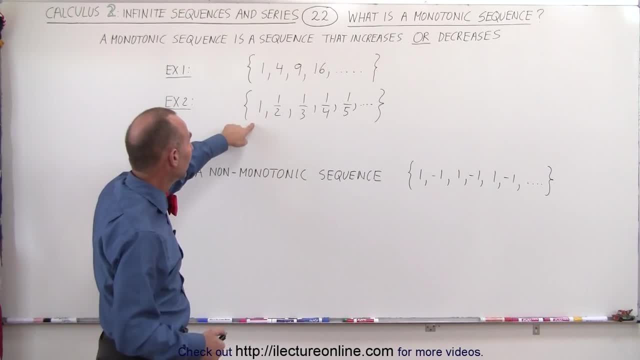 that sequence increases. Or in this case, we have 1,, 1 half, 1 third, 1 fourth, 1 fifth. so it's 1 divided by 1, 1 divided by 2, 1 divided by 3, and so forth. That's a decreasing sequence. 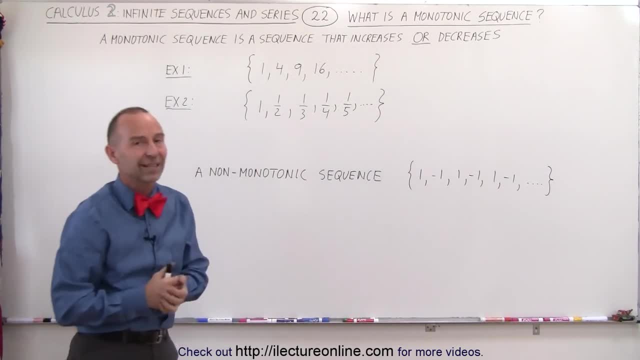 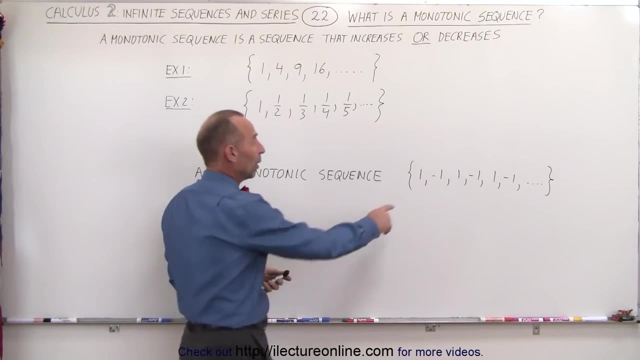 Both of those sequences are considered monotonic sequences. An example of a non-monotonic sequence is a sequence that doesn't increase or decrease. Here it's 1, negative, 1, 1, negative 1, 1, negative 1, and so forth. It keeps flipping back and forth between 1 and 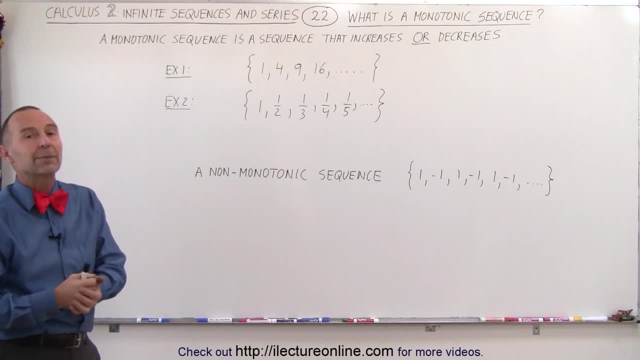 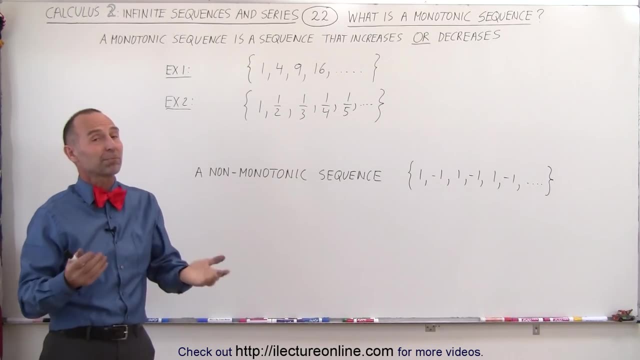 negative 1 and never converges or diverges to any particular value. So in this case, this is a non-monotonic sequence. and these are two examples of monotonic sequences. It's as simple as that. How long did that take? 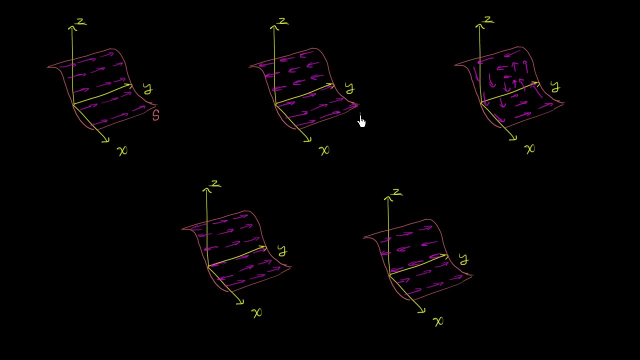 So I've drawn multiple versions of the exact same surface- S, five copies of that exact same surface- And what I want to do is think about the value of the line integral of f, dot, dr, where f is the vector field that I've drawn in magenta in each of these diagrams.